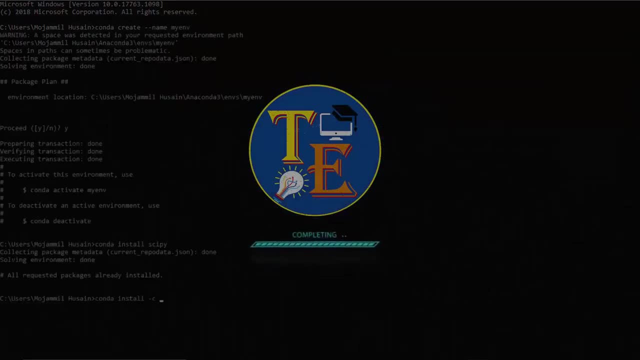 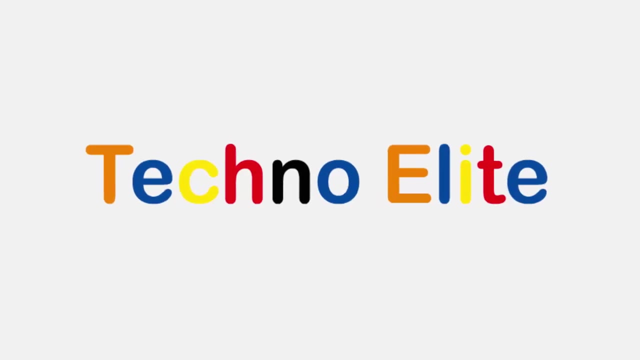 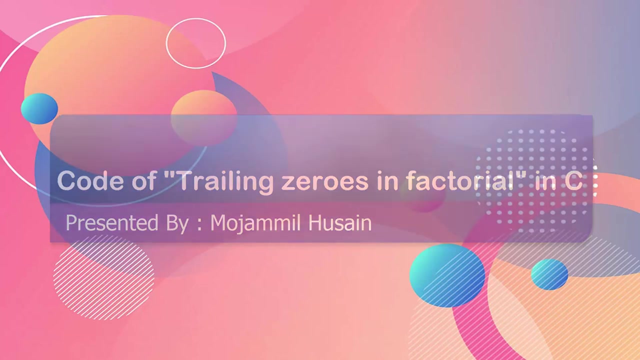 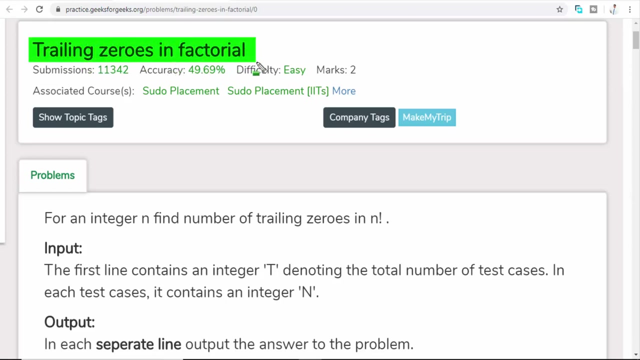 Hello guys, my name is Mujambil Hussain. Today I will demonstrate you about how to find trailing zeros in any factorial number. The problem statement is: for an integer and find number of trailing zeros in n factorial. In n factorial we have to see how much zero is behind We. 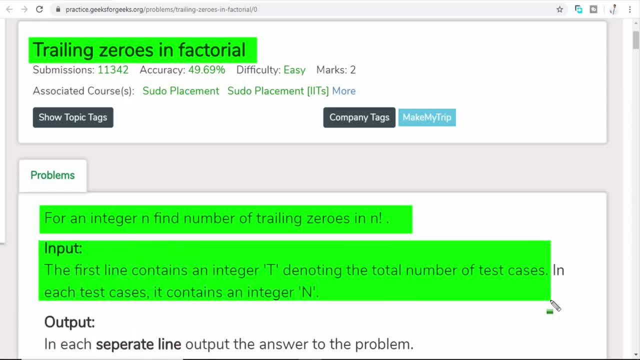 have to print. that Input is given in the form of the first line: contain an integer t denoting the total number of test case. In each test case it contain an integer n. In our first line it is for test case and in second line it is given for number of. 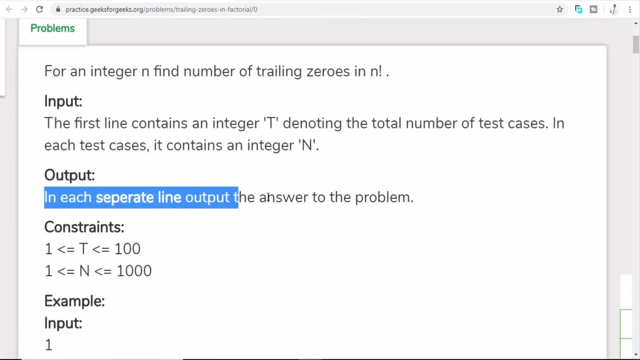 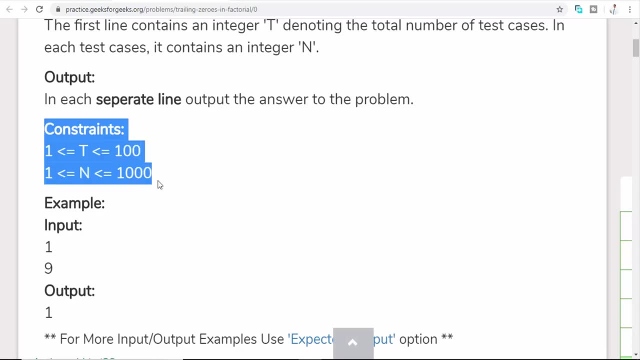 factorial. The output is generated in the form of: in each separate line output. the answer to the problem: We have to generate one output in each line. Here the constant is given, The limit of t is 1 to 100 and the limit of n is 1 to 1000.. Here the example is given. 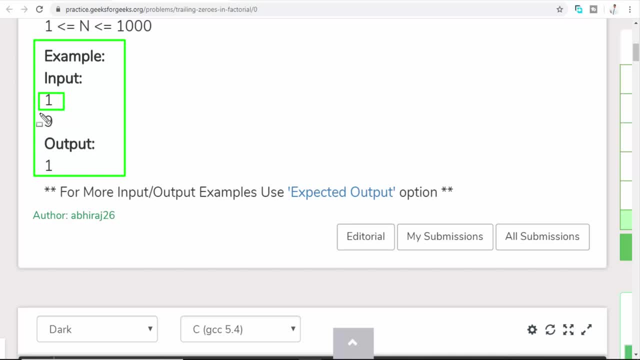 In the example the first input is a test case and second input is a factorial number And that factorial number it will generate as output 1. That means the 9 factorial have 1.. First of all we go through one slide and we will understand about how we can find. 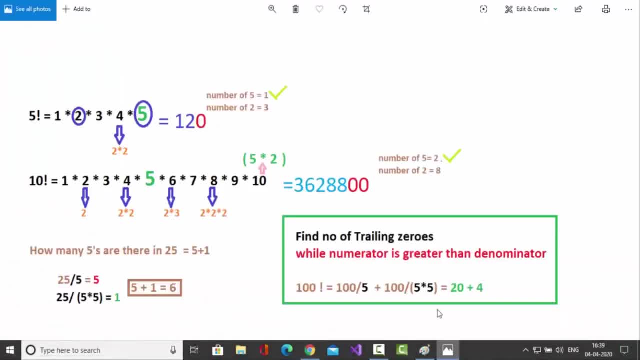 the trailing zeros of any factorial number. In this slide we will see how to find the trailing zeros of any number. So we have taken an example of 5 factorial. First of all we will see what we get by expanding 5 factorial. Expanding: we get 1 into 2, into 3, into 4, into. 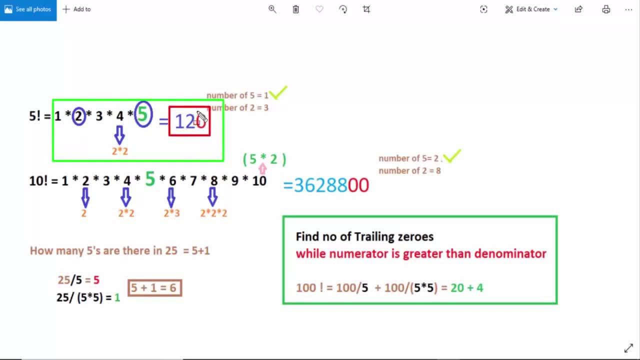 5. And if we calculate it we get 120.. The number of trailing zeros of any number is 1 into 2, into 3, into 4, into 5.. The number of trailing zeros of any number is 1 into 5.. And if we calculate all of it we get 120.. So here, the following number is the very 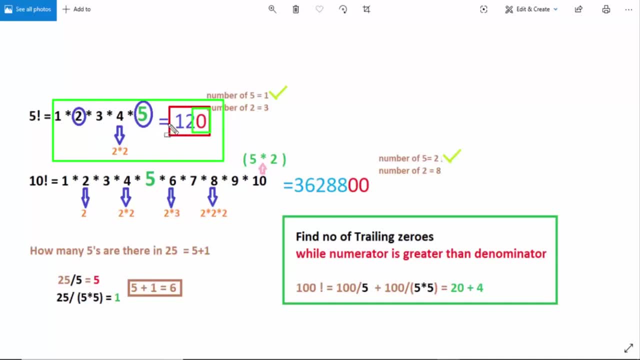 suffix of EV 10168.. We calculate the sum of the trailing zeros of any number, conten. number of point. The first thing we do, we will see that how many this zero? The trailing zero of a, is the number of points. 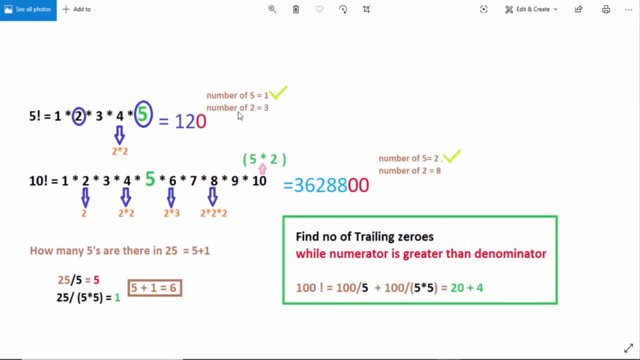 So here we will see that how many trailing zeros trailing zeros are there. 1 is there, So we have to find out how much The trailing zeros are. We have to find one. Only 1 is there, So we will first see that how many time is 2? 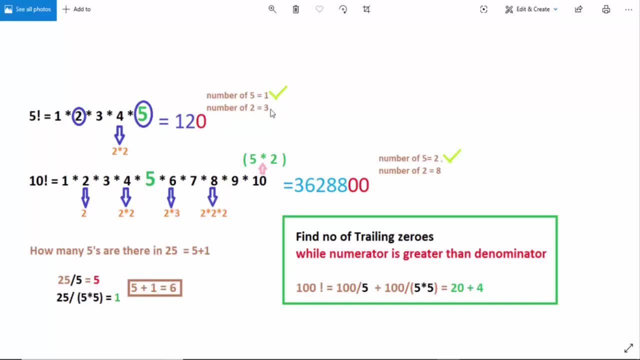 and when 5 is used. So 2 is our 5, 2 is us. so 1 is stereo, 2 is 2 is here and here is 1 is one. zero is 5 factorial each 1.. We got 1.. Why? 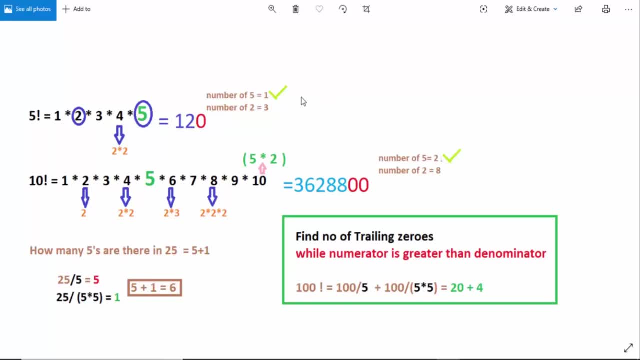 do we subtract 5 and 2 and why don't we take any other number? That's why we take 5.2, because in any multiplication, if we multiply 5 into 2 by 10, then it goes back and adds up to 1 zero. 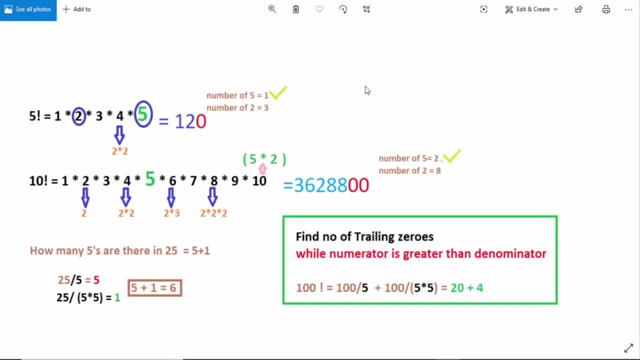 That's why we have to find the zero at the back And whenever 5 comes, whenever 5 comes and whenever 2 comes, if we find it, then in the least number we will find it. That will be our trailing zero. 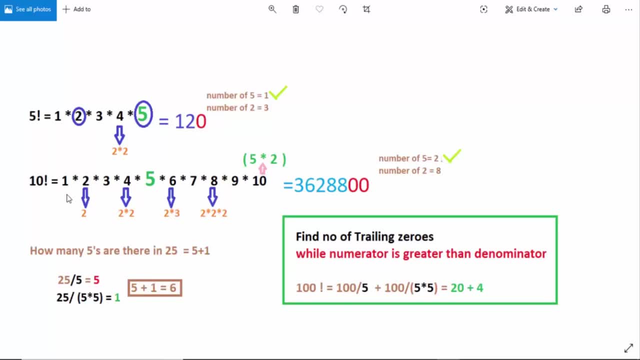 And we will see the next example in 10 factorial. If we expand 10 factorial then we will get 1 into 2, into 3 to 10. In this we will see that if we calculate it we will find 3628800.. 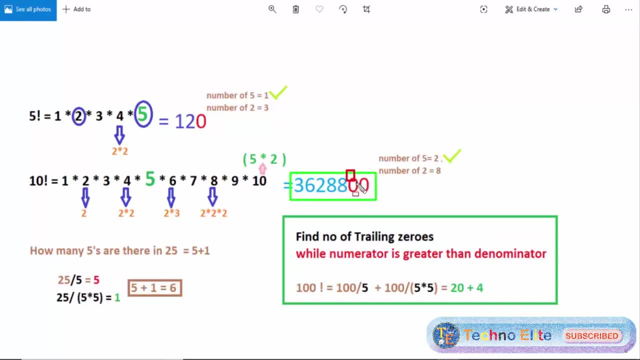 So here our trailing zero is 2.. We have to subtract it. We will first subtract it here. We will see how many times 2 has come and how many times 5 has come. So we subtracted here how many times 2 has come. 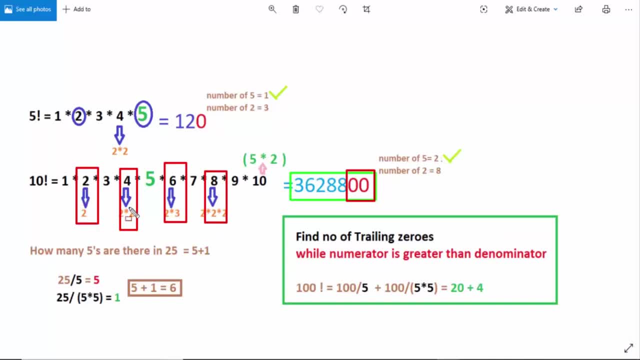 So one comes from here, 2 has come from here, 1 has come from 6, 3 has come from 8 and 1 has come from 10, So 1, 3, 4, 4 plus 1 is 5, 5 plus 2 is 7. 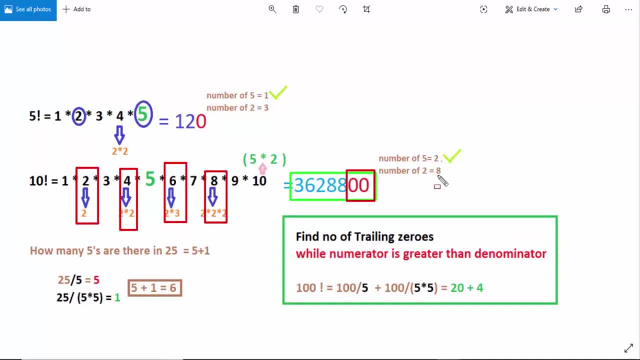 7 plus 1 is 8. Number of 2 is equal to 8 and number of 5 we have to subtract. So 1, 5 has come from here. 1, 5 has come from 10, So number of 5 is equal to 2. 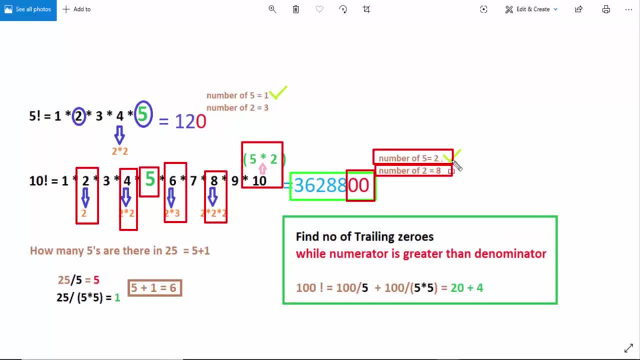 Who is in the least? number 5 is. So we got the trailing zero. How much is it? What is it? What are the trailing zeros? Now we will see an example. We will see the question: How to subtract it. 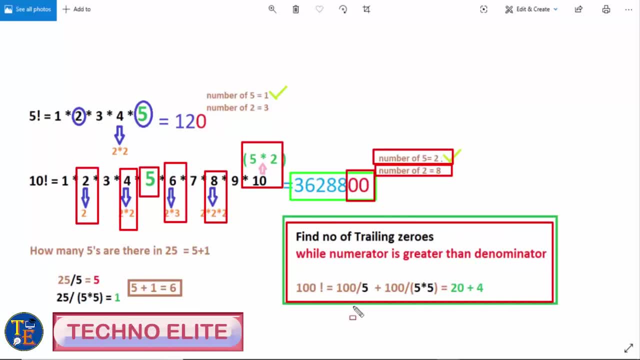 So if we want to find out 1,, 10,, 100, How to subtract it, So we will find out in the code, So we will see here that it is 100.. So if we divide from 5 in 100, So we will first get. 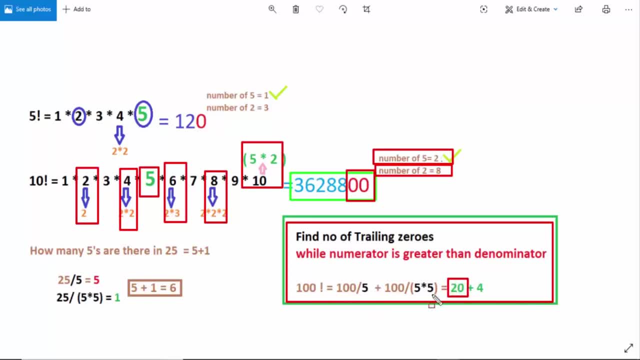 How many trailing zeros are there? Then if we divide by 5 into 5, You will do multiple 5. So then we will subtract. 4 will come from here. So 20 plus 4 is equal to 24. How long will we do this? 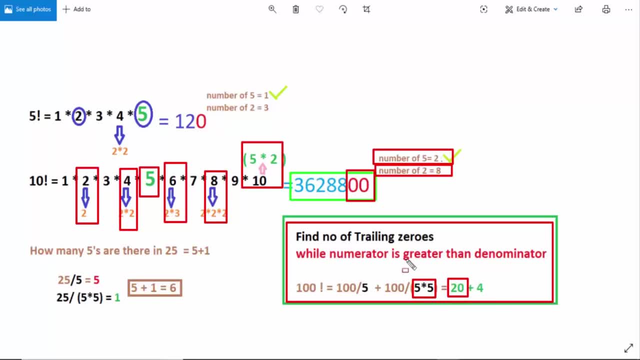 Multiply by 5 While the numerator is greater than the denominator. Until the numerator is greater Will be more than the denominator. Till then we will do So. here we got 24, 100. factorial trailing zero is 24. Here is the question. Let's see this: How many 5 are there in 25?? 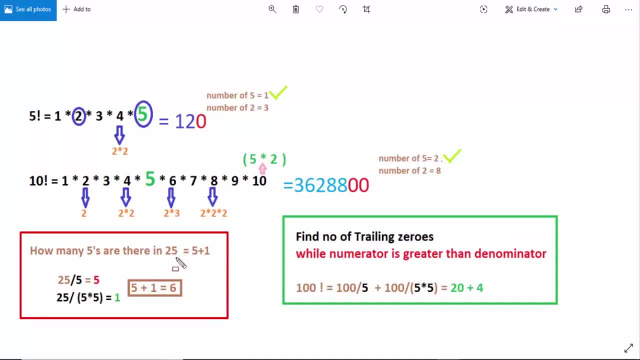 How much 5 is there in 25?? So we will first subtract it: 5 divided by 5 is equal to 1, And then 5 is left. So if you do 5 divided by 5, Then 1 will come. So 5 plus 1 is equal to 6. 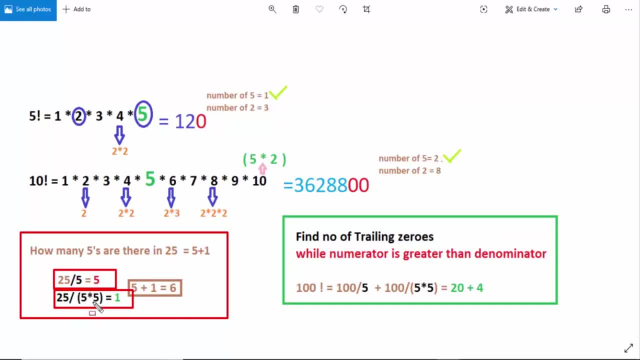 Here we have said: If we want to write a code, Then we will multiply from 5 to 1 In the second number, Not more than the denominator. Not more than the denominator 25 is equal to 25. So we got 1 here. So 5 plus 1 is equal to 6. 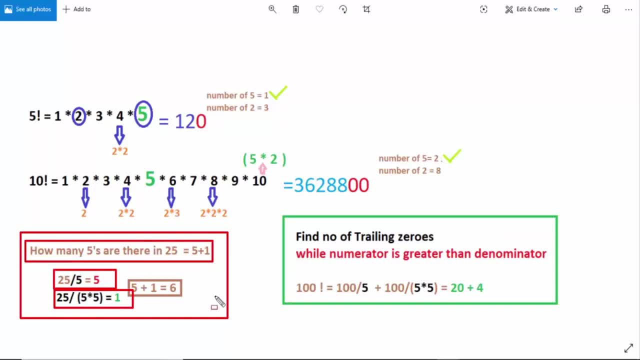 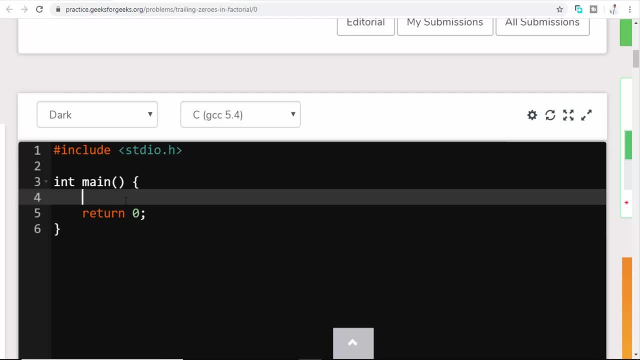 How many 5 are there in 25?? 6 5 are there in 25. And now We are going to write the code In C language. First of all, we will take the input of T Test case as T, And now we use for loop. 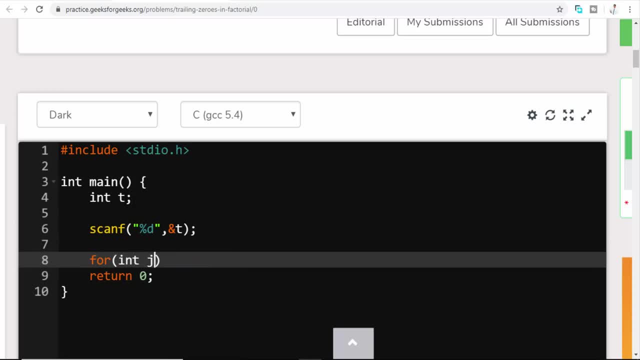 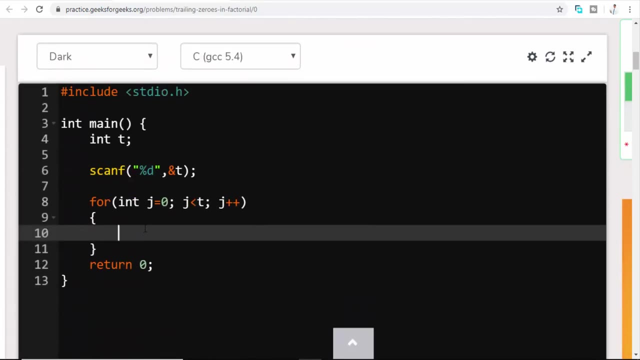 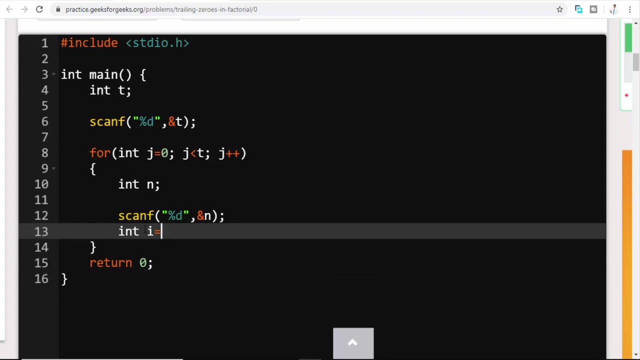 That test case J is less than T, J plus plus. And the next input is The number factorial. We will initialize it As n And we will take the input In n And also initialize i is equal to 5 And count is equal to 0 And also initialize.